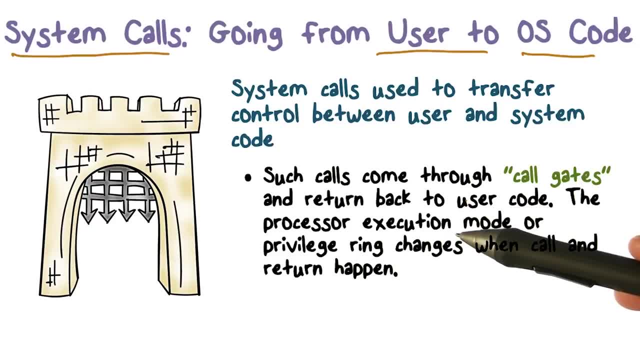 Okay, this is defined by the application programming interface or the API that your operating system provides. So you have these calls and these calls have to come into the operating system in a controlled fashion. okay, So we said these calls are different than regular calls. 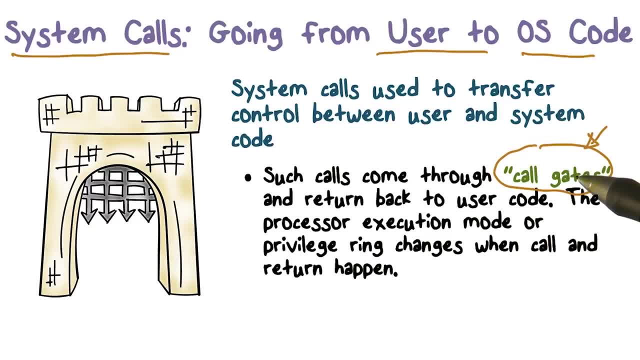 They have to come through what is called used to be called call gates. These are sort of special ways in which you can enter from user to- it's a defined way, transition from user to system level. You come through these call gates. 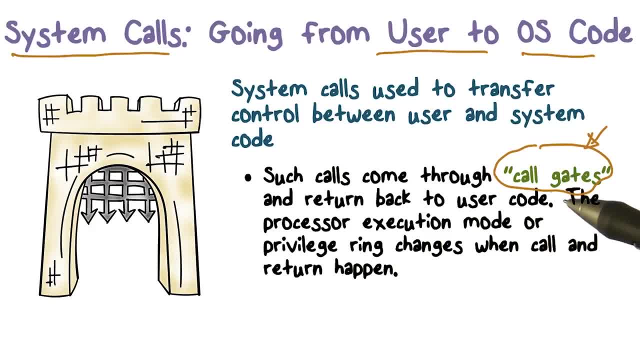 And what happens as a result of that is: well, we know that it's a call, so we're going to return at some point. So we have to keep track of where we're going to return and the user code once the system call completes. 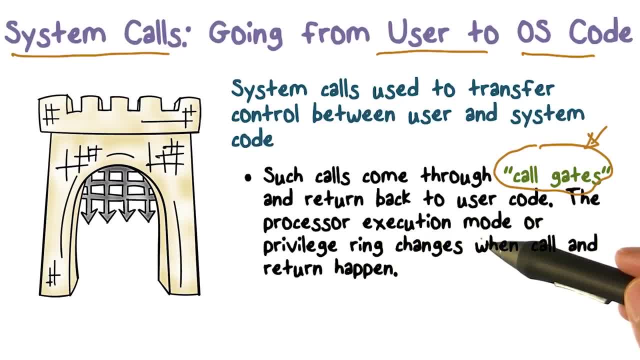 But the processor execution mode has to change as a result of that, isn't it? We're going from user mode to system mode, So the pool is ring or the mode is going to change And we actually going to be able to. we'll have to change some memory mappings. 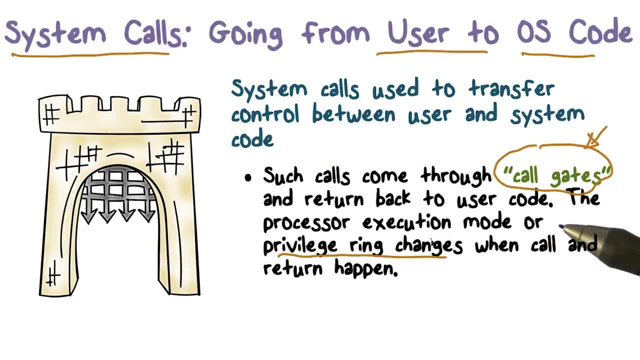 data structures that keep track of those, Because we're going to be able to access memory now that we couldn't access before. So some registers have to be saved, others have to be loaded and things like that. So all that work has to be done. 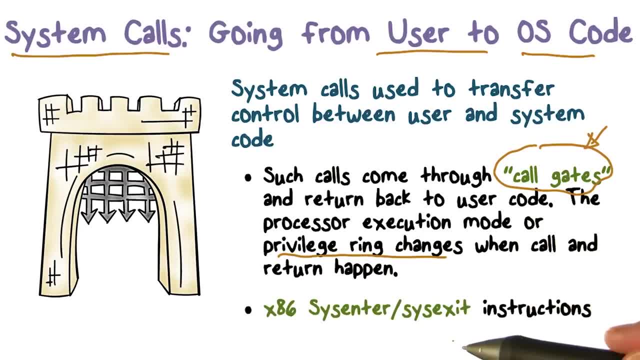 So now we are executing in a different protection domain. In fact, this used to happen through sort of an interrupt or a trap into the system from user mode, But in x86, we actually have explicit instructions. This is different from your regular call return. 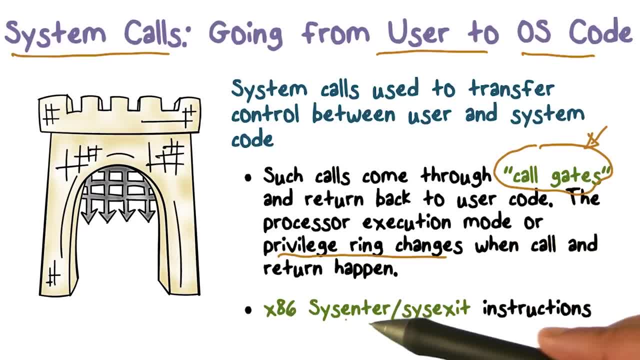 These are: execute a system call, that's sys enter. Enter the system or the operating system And when you're done you return by doing this, another special instruction called sys exit. So there are these instructions that help you implement this system call that we're talking about. 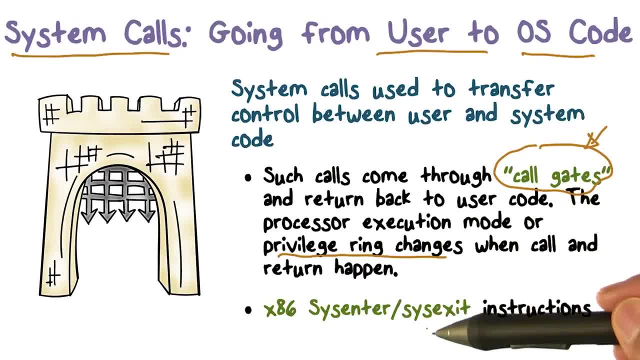 Keep in mind that they are more expensive, because now we are using- we're doing this work that we're going to have to- we had to check what kind of call it is Arguments that are being passed. save information when we come back. 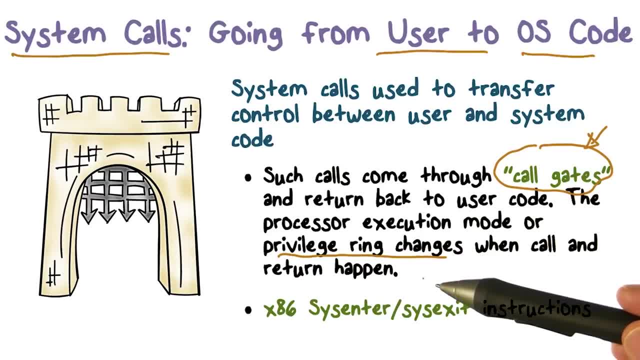 And change memory mapping so we can access things that we couldn't before, Use the special instructions rather than the regular ones, and so on. So that's what makes it costlier or more expensive.